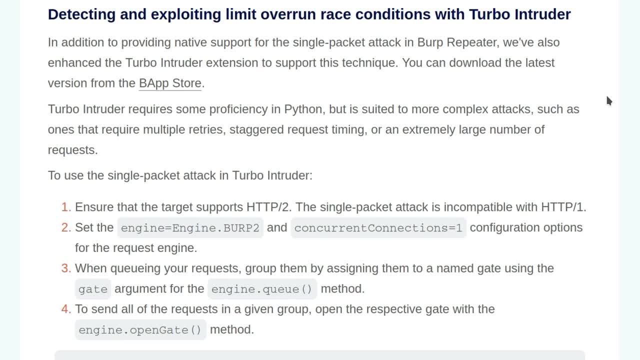 Detecting and exploiting limit overrun race conditions with Turbo Intruder. In addition to providing native support for a single packet attack in Burp, Repeater Ortsfigure has also enhanced the Turbo Intruder extension to support this technique, And we can download the latest version of that from the Burp App Store. 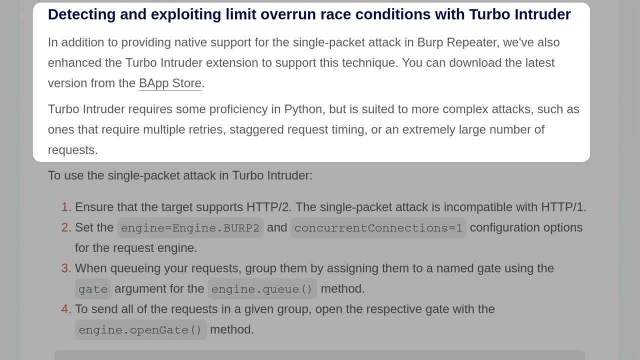 Turbo Intruder requires proficiency in Python, but is suited to more complex attacks, such as ones that require multiple retries, daggered request timing or an extremely large number of requests To use a single packet attack. in Turbo Intruder, we can follow these four steps. 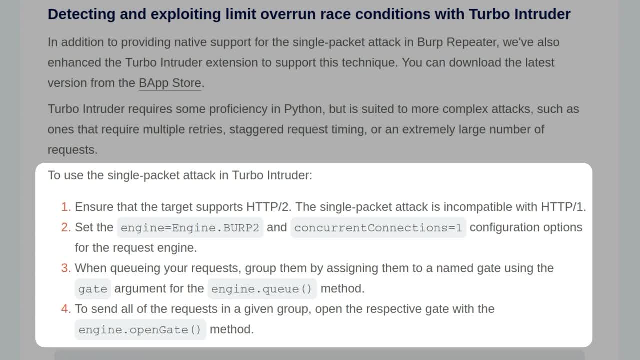 First is to ensure that the target supports HTTP2, as the single packet attack is incompatible with HTTP1.. Second, we need to set the engine to equal engineburp2 and the concurrent connections to 1 in the configuration options. Thirdly, when queuing the requests, we need to group them by assigning them. 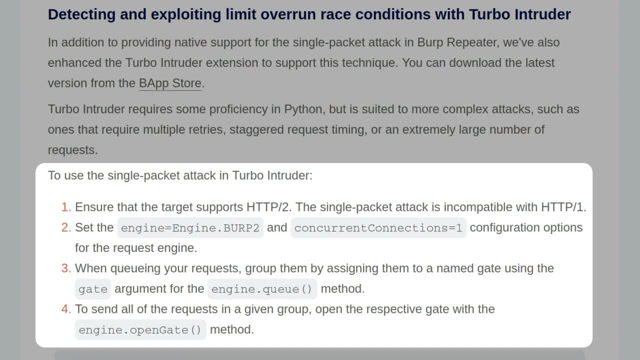 to a named gate using the gate argument for the enginequeue method. And finally, to send all of the requests in a given group, we need to open the respective gate with the engineopenGate method, And here we have an example of that. 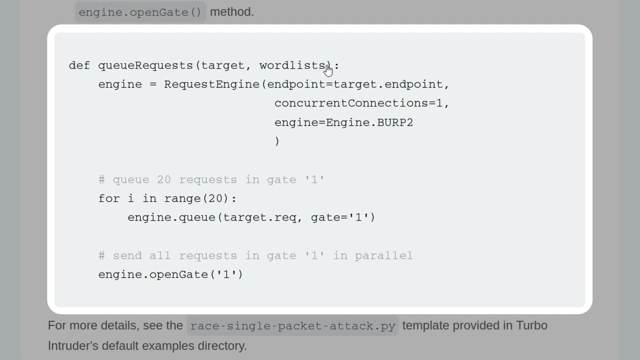 So you can see we've got this function- queueRequest- which takes a target and wordless, And then we set the engine configuring the options as advised. So we need concurrent connections to equal 1 and we need the engine to be engineburp2.. 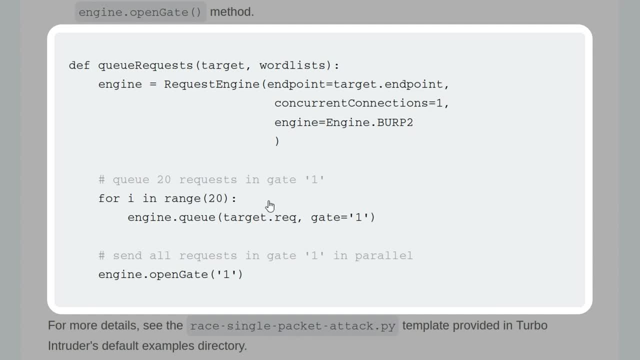 And then, in this case, we are queuing 20 requests for gate 1. And then, eventually, we're going to open that gate. For more details, we can see the raceSinglePacketAttackpy template, which is provided in Turbo Intruder's default examples directory. 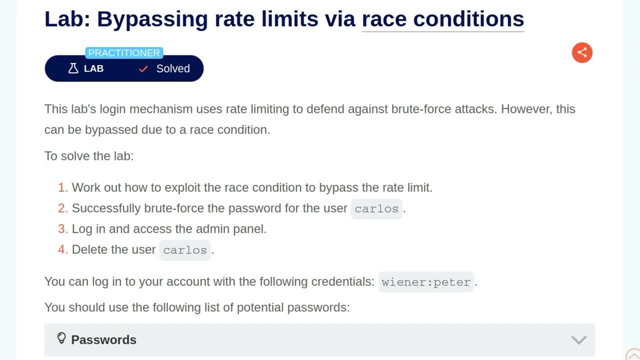 So that brings us on to the practical lab: bypassing rate limits via race conditions. The description says this lab's login mechanism uses rate limiting to defend against brute force attacks. However, this can be bypassed due to a race condition. To solve the lab, we need to work out how to exploit the race condition. 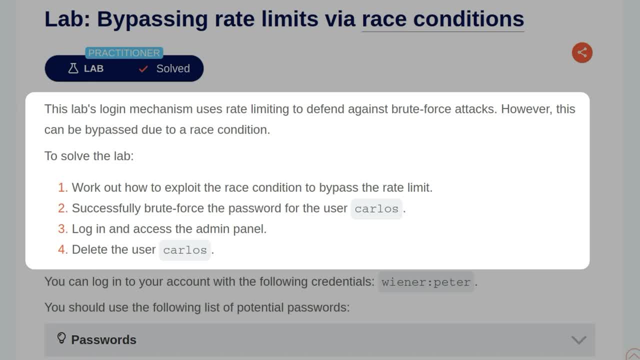 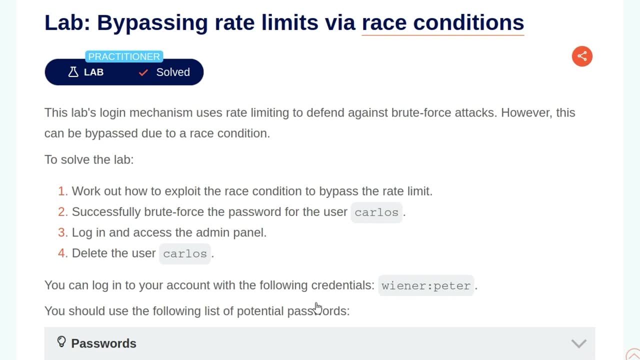 to bypass the rate limit successfully, brute force a password for the user, Log in and access the admin panel and then delete the user. Carlos, As usual, we're given some credentials that we can log in with, And this time we've also been given a list of potential passwords. 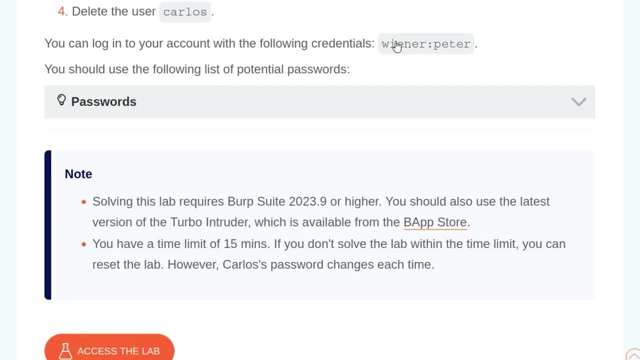 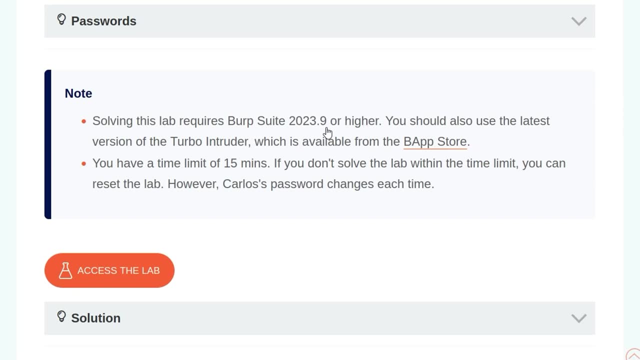 I didn't actually see this whenever I solved the lab, So you can also just use a common password list. And then there's a note which says we need to use burp September 2023 or higher And we should use the latest version of Turbo Intruder from the burp app store. 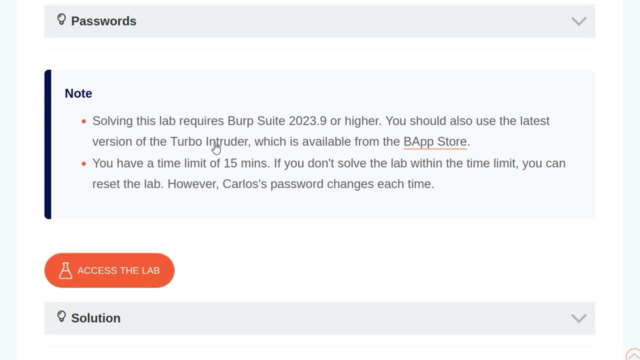 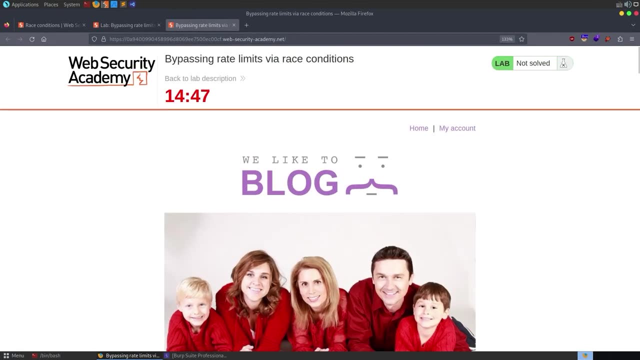 We also have a time limit of 15 minutes. So if we don't solve the lab within that time, we need to reset it, but Carlos's password will change each time. All right, so we get through to the lab. we've only got 15 minutes. 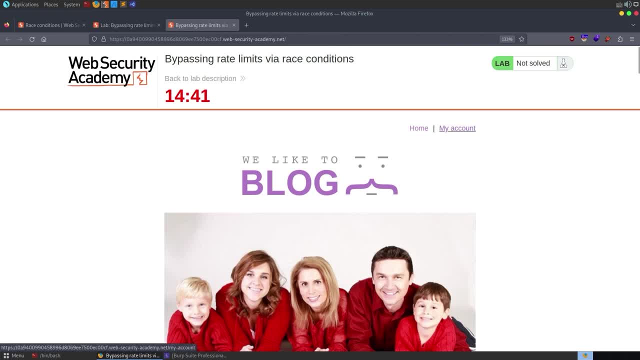 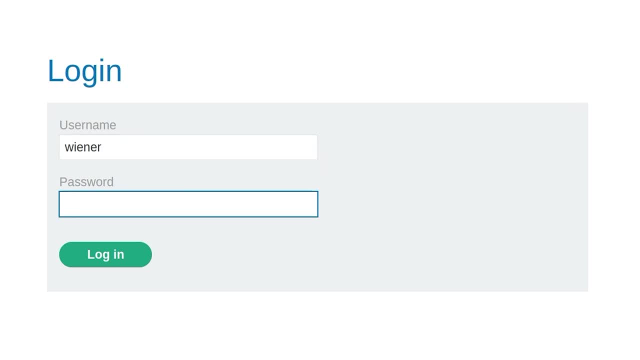 and if we get down to like three or four minutes, then we don't really have much time to test out our attacks. So let's try and move kind of quickly. I'm going to start with the user that we have the credentials for, because I don't want to lock out the user that we're targeting. 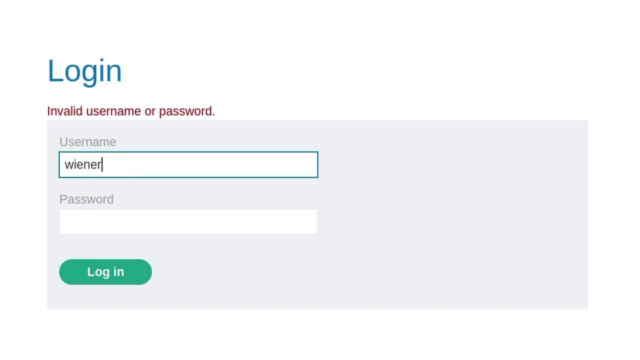 And I'm just going to put in some incorrect credentials. I guess I could have just used a shorter password. Let's do that twice, And a third time and a fourth time. I noticed then that after three login attempts we were locked out for one minute. 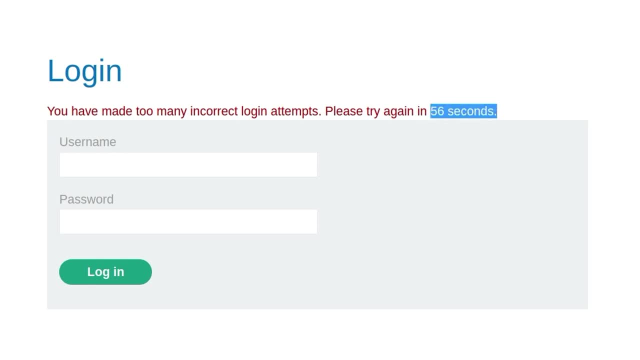 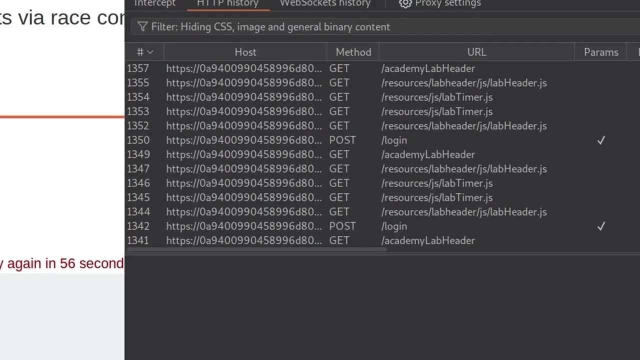 I believe this also increments. So next time we get locked out, we'll be locked out for two minutes. So that's the general process here And now. we want to go and see what happens whenever we use the burp repeater, So we want to let this reset. 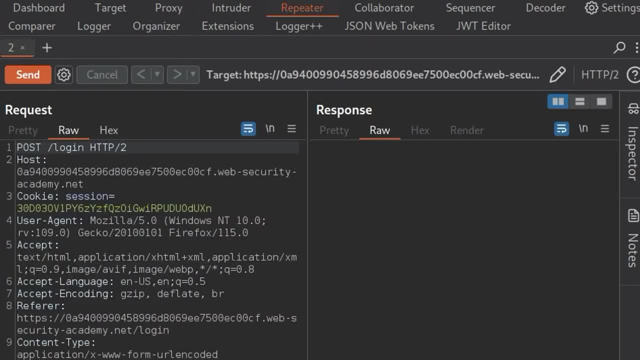 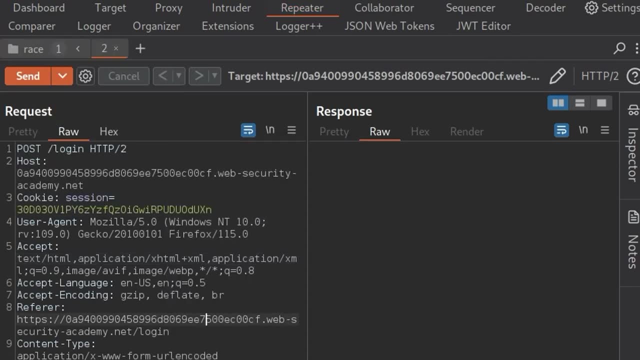 Actually let me wait for one minute, but I'll also send this to repeater. We'll get this ready and we can do a group. first of all, Add to a group, I'll call it race, And then I'll do control and R to create. 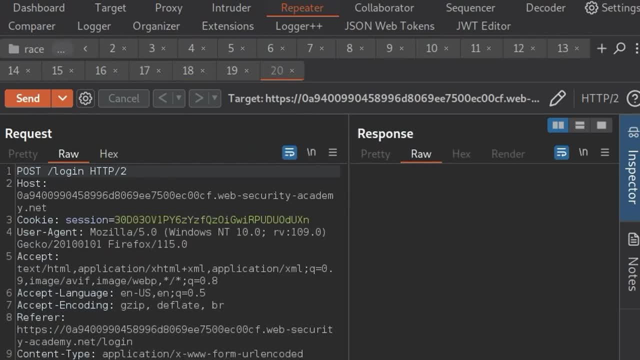 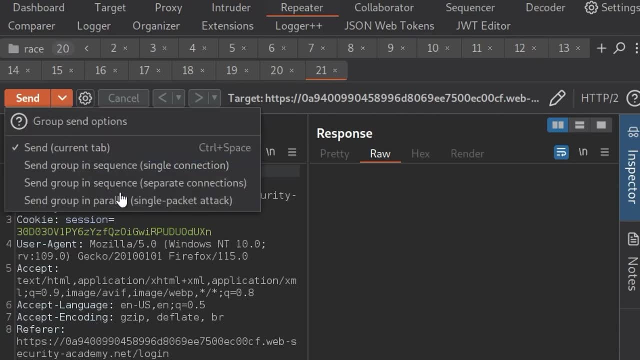 We'll go with about 20 tabs again. Okay, so I waited for over a minute, So we are now clear to try this again, And this is the probe page where we would normally try and find out what happens when we send this in a sequence of separate connections. 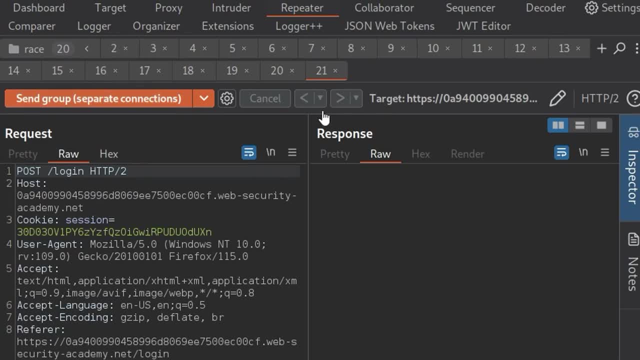 And if I click that, it's basically going to send each one of these 20 requests one after another using separate connections. I'm not going to do that, because what we're going to see is what we just saw when we did this manually. 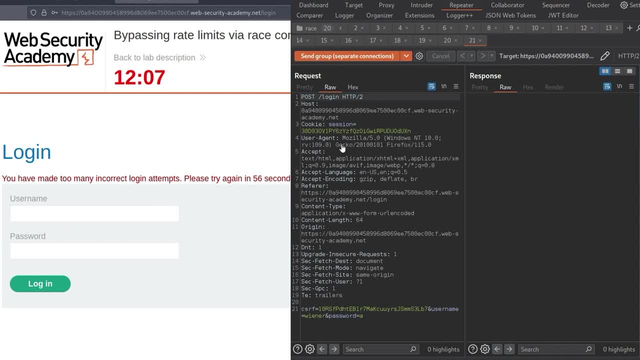 Namely that The first three requests will come back and say incorrect password And then every request after that will come back to say that we've had too many login attempts and we need to wait this period of time. So I'm not going to do that. 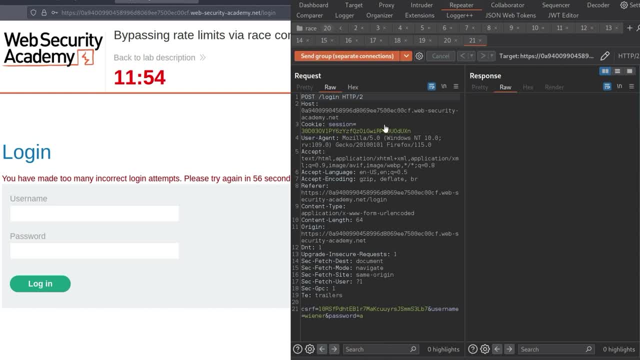 But this is how you would generally approach these. You would go and find some kind of functionality. You see how it behaves whenever you send multiple requests as separate connections in a sequence, And then you'll do the exact same thing again, but you'll send them in parallel and see how it responds differently. 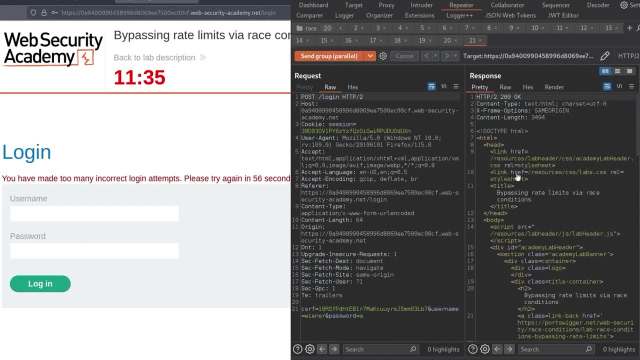 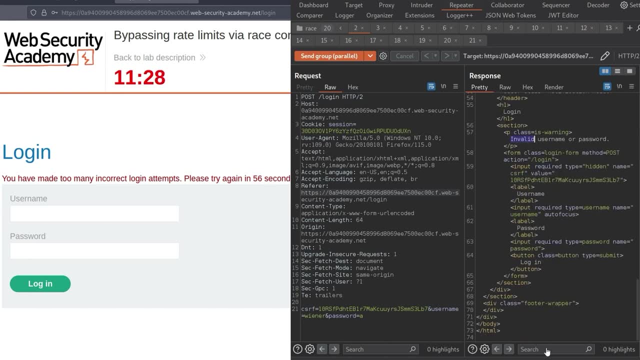 I'm just going to jump straight to that stage, Because we did already do the manual lockout, And then we just go through each one of these responses and see what we've got. So we can see with the first one we have invalid username or password. 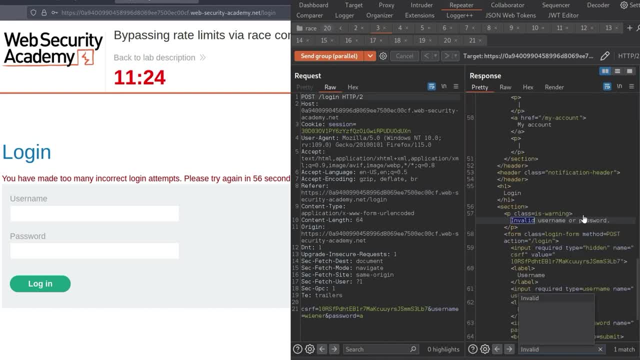 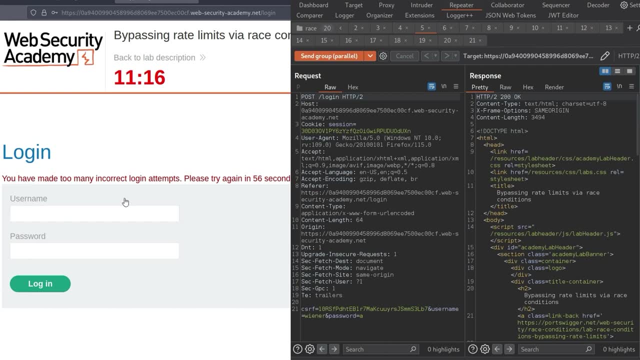 We can actually do a search here as well, Although it's kind of annoying that it resets each time. So there's our first three: All invalid, as you'd expect. Now, based on what we saw when we sent these requests one after another, we would also expect this to be. 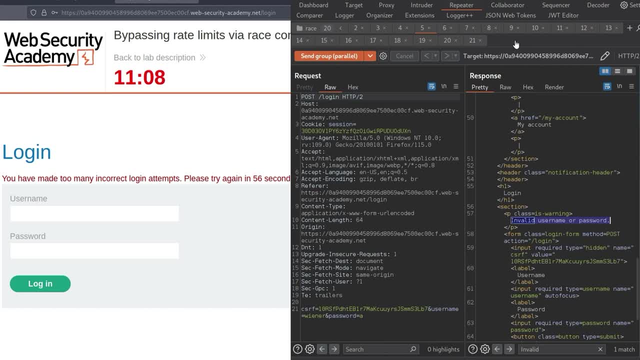 Sorry, we would expect this one to be a lockout, But it's also invalid. And if we go on to the sixth one, That's also invalid. And if we go on to the seventh one- And I think you're getting the idea- 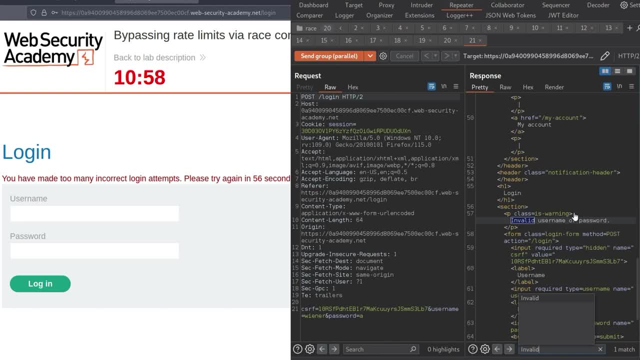 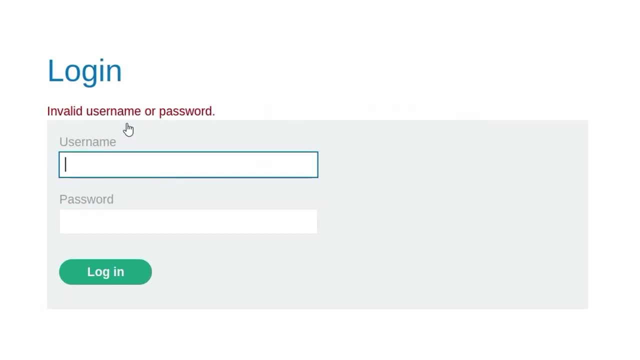 We can go to. let's go to the 20th tab. And it also has invalid username or password, Which means even though the lockout will have occurred. In fact, if we go here and just try an incorrect credential, Okay, I think the time might have reset, since I did that. 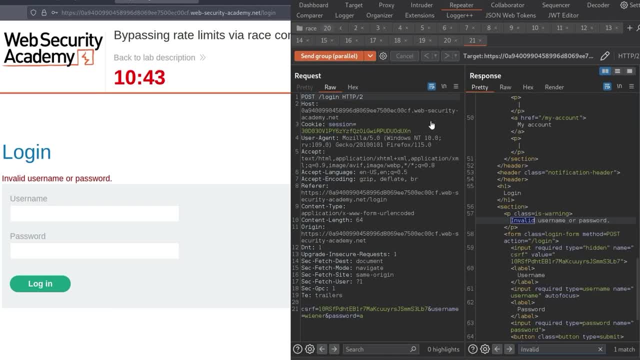 But it will still lock us out. It just means that the 20 attempts that we already sent were all successfully returned, So we were able to find out whether those 20 passwords that we tried Were valid, Even though we should be locked out after three attempts. 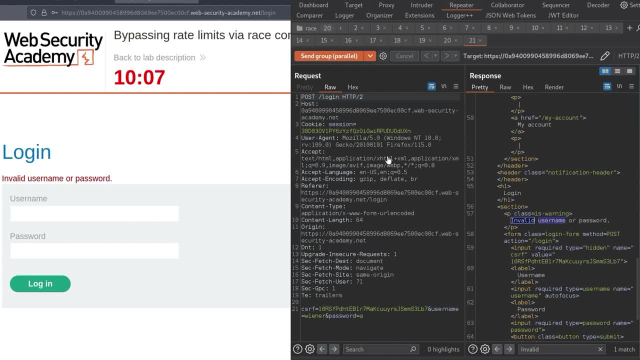 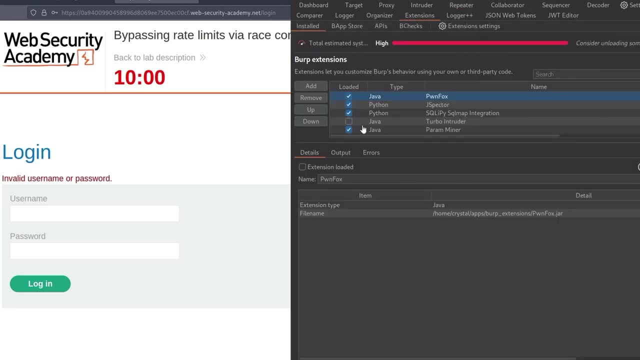 So the next thing we'll do is send this through to the turbo intruder, So we can just take one of these requests And I'll go to extensions, And then I don't actually have turbo intruder, So just make sure that you have the extension installed and activated. 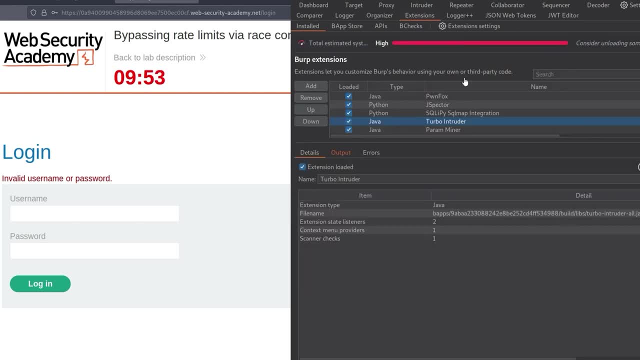 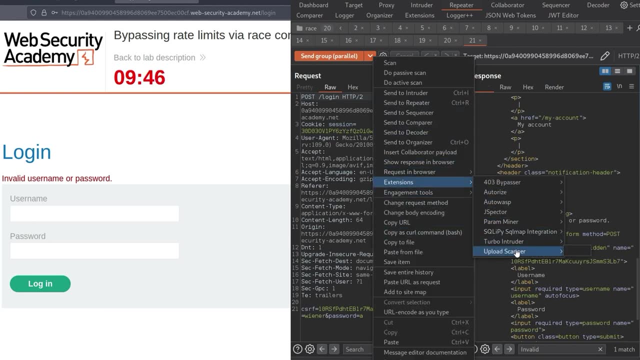 I'm going to activate it now. Activated without issues. So let's go back to our repeater, Or you can go into proxy, Just wherever you can find this request, And then we can send it to the turbo intruder And this opens up. 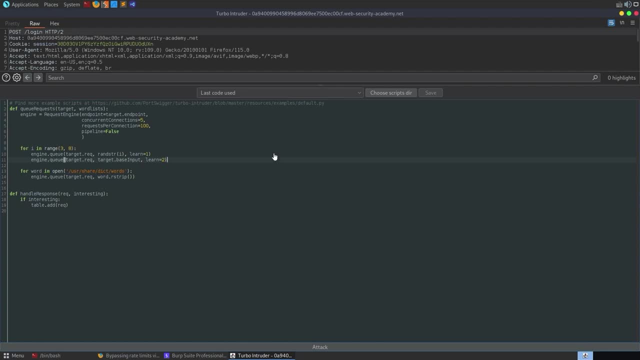 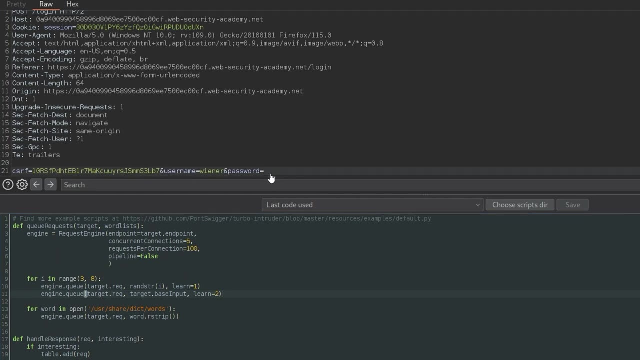 I can't actually increase it. I can't actually increase the text size here. It's just whatever is used for burp overall. But essentially we have our request at the top And we want to say what we want to update here. So in this case we're going to be looping through passwords. 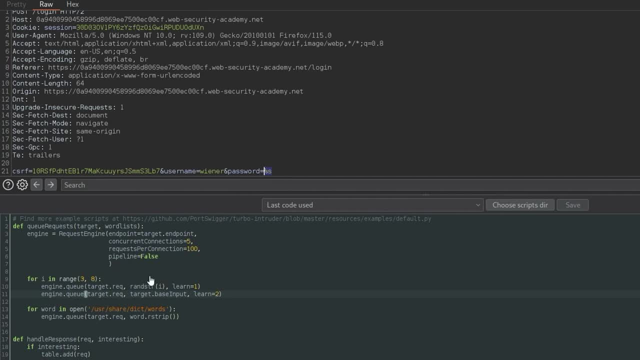 So I'm going to put the percentage S there To denote that's the value. we want to be replaced with each of the words in the word list. And here we have the script. So I'm going to change this to the single packet attack. 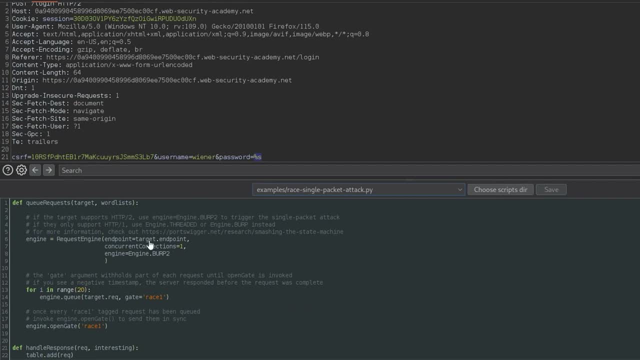 That we saw in the port swigger notes And notice then That the concurrent connections are set to one And we've got this burp2 engine being used. That was one of the requirements And we also have this gate, So essentially we're queuing 20 requests into this gate. 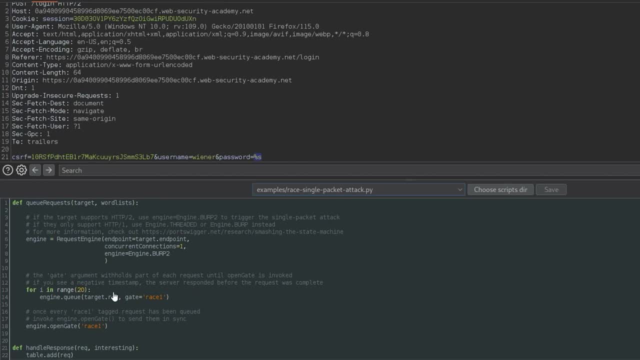 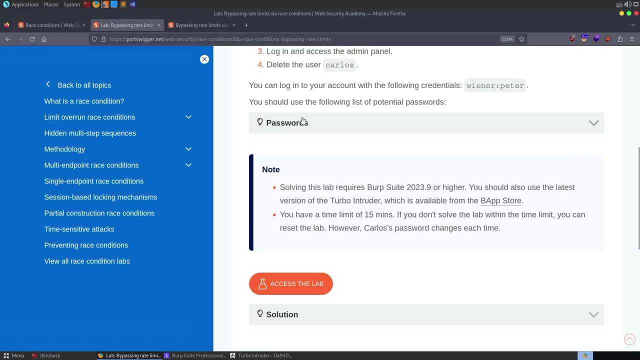 And then at the end we're going to open the gate So they all get sent at once. Now we need to provide the word list that we're going to use, So I'm going to go back to our lab And grab these passwords. 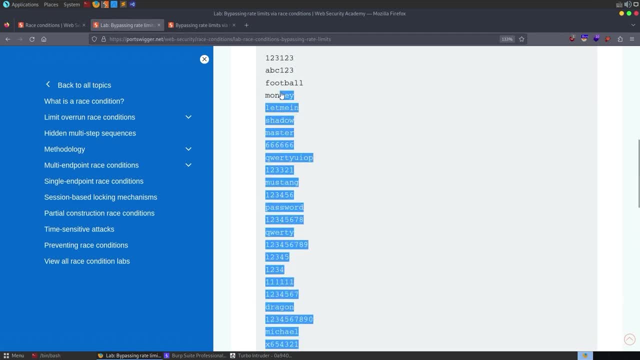 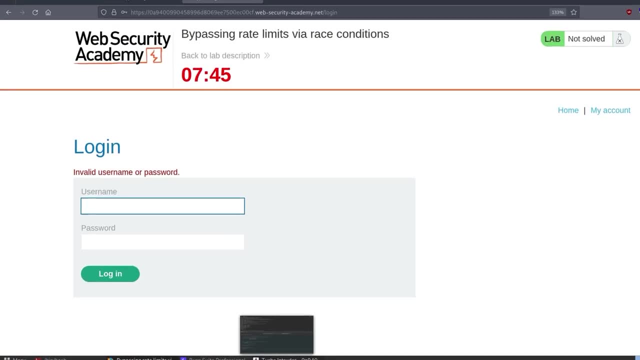 Actually the first time I solved this. I just used a word list of 200 passwords And it worked first time. But that isn't guaranteed And I don't want to waste too much time in the video, So I'll talk about this at the end. 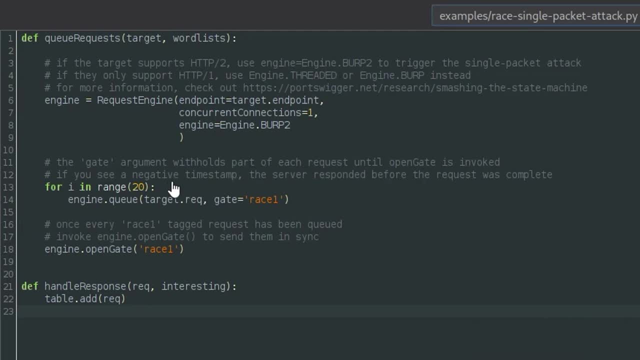 But for now I've copied those into the clipboard And actually what we can just do is say that our words are equal to. In fact, what I'll do is do for i in, And instead of range we'll say word list dot clipboard. 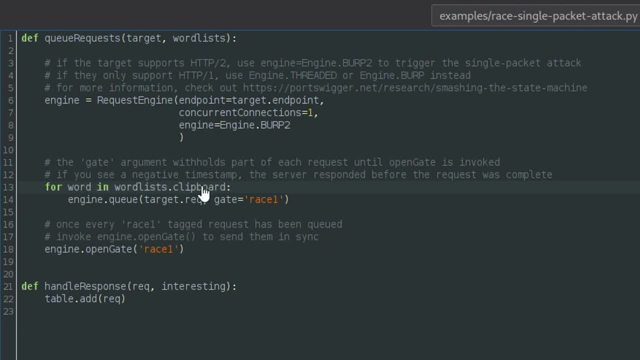 And I'll change this to word, So for word in our word list. Let us queue a request And then you want to supply the word there as well in the queue, And I believe that should do it. We can also use this handle response. 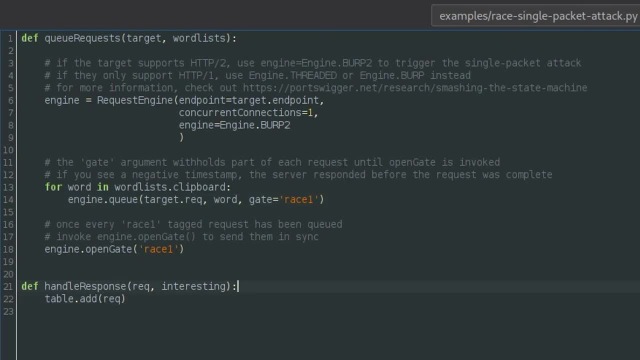 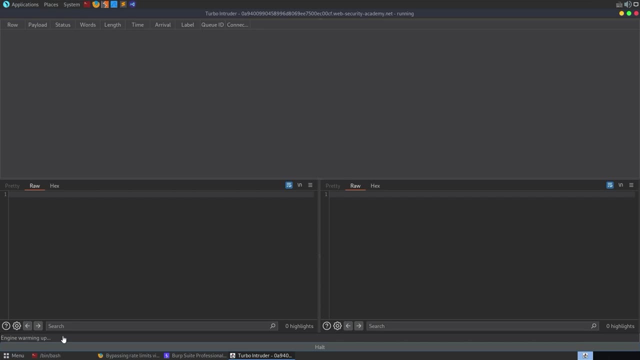 I'll talk about that at the end, So that we don't waste too much time. for now, Change this to Carlos And we'll try and do the attack. The engine is warming up, apparently, And there we go. So it sends off all the requests at once. 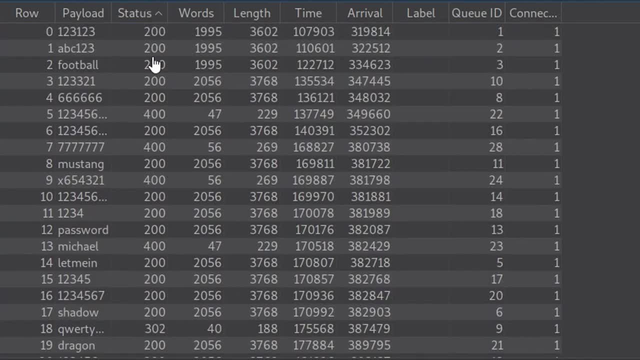 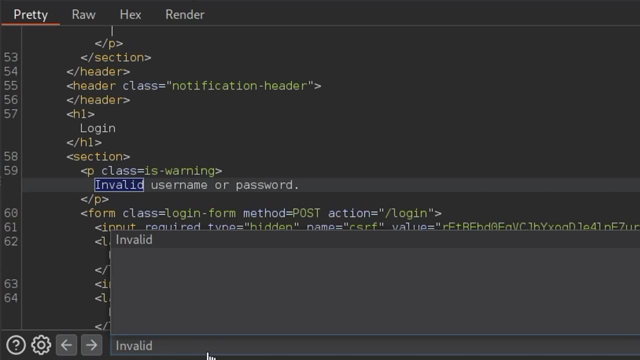 We get back all the responses at the same time And we want to basically go through and have a look at the status of these. Or it could be you look for some keywords, So maybe we look for that invalid message And then we look for one that doesn't have it. 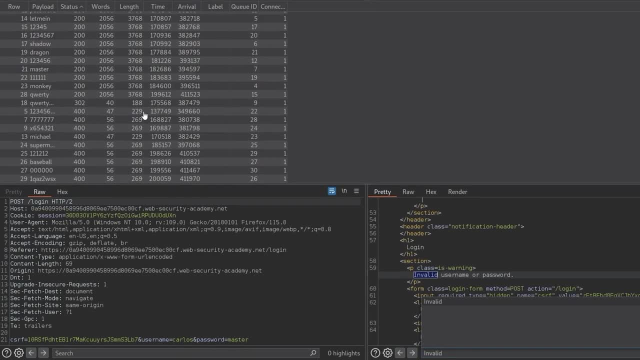 Or we look for one that has successful Logged in or something like that, But in this case we actually see there's only one request that has a 302.. That's 302 found. It's because it successfully logged us in And it's redirecting us to our account. 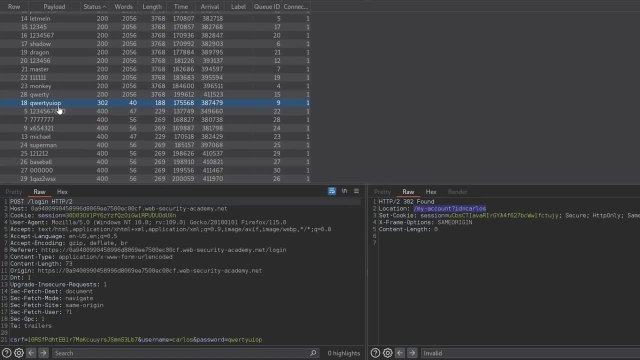 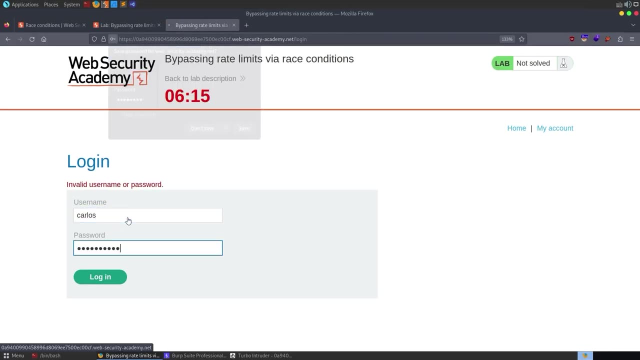 And that means we found the password. So the password is qwertyuiop. So I'm going to take a copy of that And I'm going to go back to our lab. We might still be locked out, But let's try it. 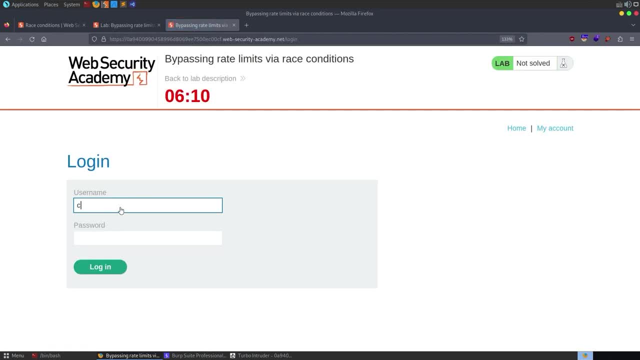 Okay, Invalid CSRF token. Let's try it again. Yeah, Too many incorrect attempts, But it's going to reset in five seconds. And there we go, We log in And now we can go and delete our account. Where is it? 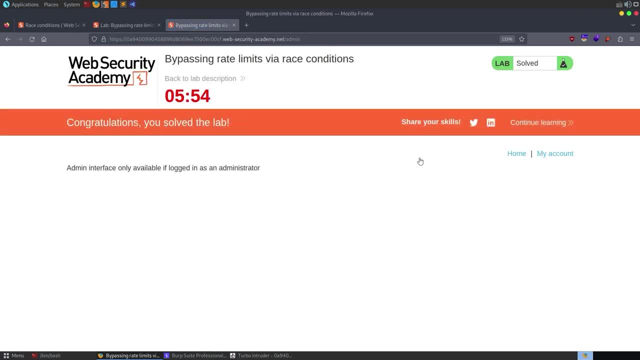 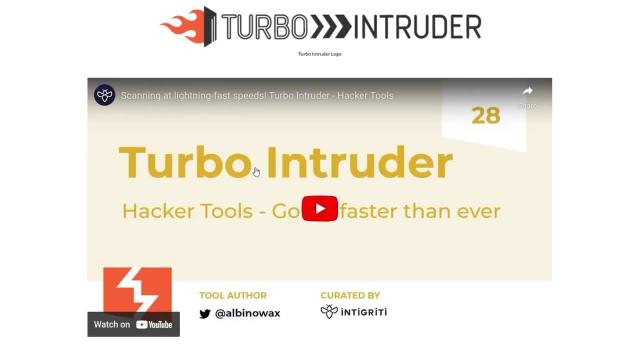 Admin panel. Delete the user Carlos. And there we go. We've solved the lab. I've just moved over to the Integracy blog as well. We did a post a while back on how to use Turbo Intruder, And it talks a little bit about some of the configs. 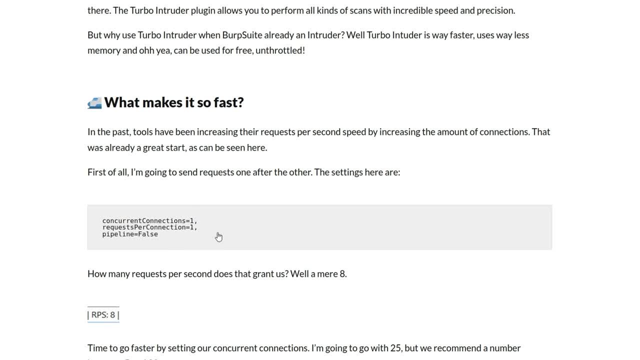 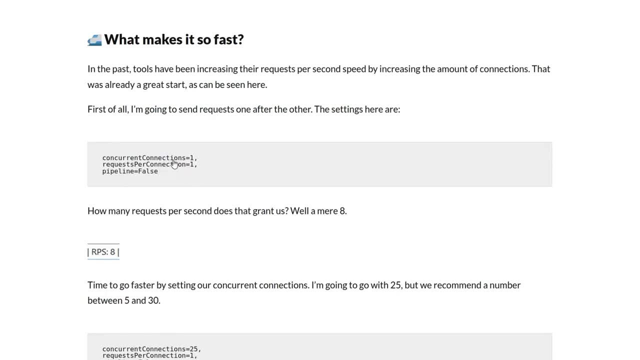 So we just mentioned there that we can't change our concurrent connections. But just in case you haven't used Turbo Intruder before, You want to learn a bit more about it- If you were just doing some standard Brute forcing- Assuming you don't have the Pro Burp Suite- 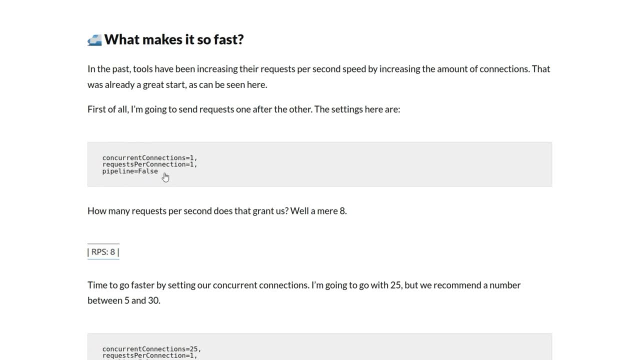 That has an unthrottled intruder. You probably want to use this Turbo Intruder Because it's free And you can just write a Python script yourself, But by default It will only give us eight requests per second. However. 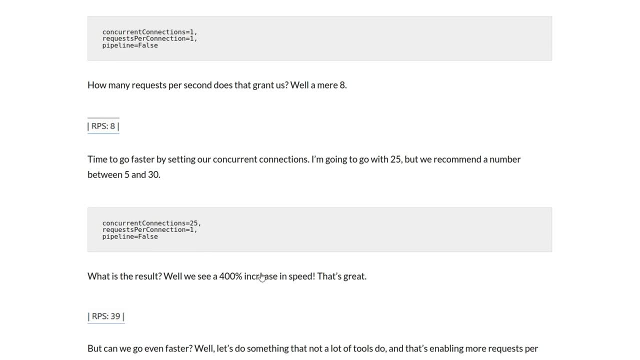 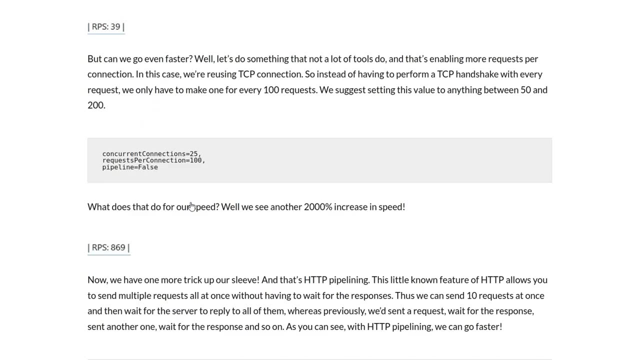 By changing the concurrent connections to 25. We get a 400% speed increase, Although we can't do that for this single packet attack. And if we want to go even faster than that, We can also increase the request per connection. So if we change that to 100. 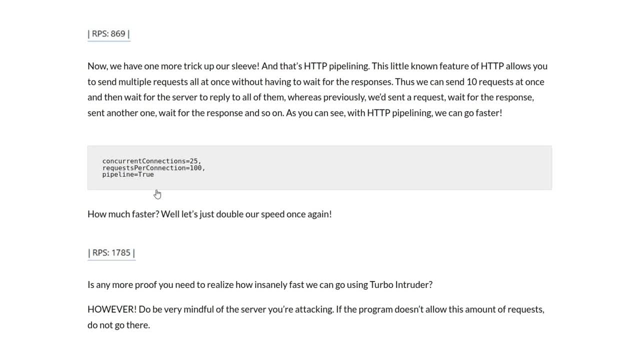 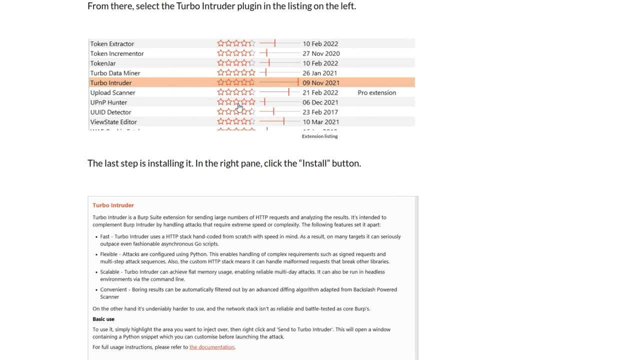 We'll get another 2000% increase in speed, And we can also use pipelining, Which will double our speed once again. So just worth bearing in mind, Just in case you want to use this more often in general For web pen testing or bug bounty. 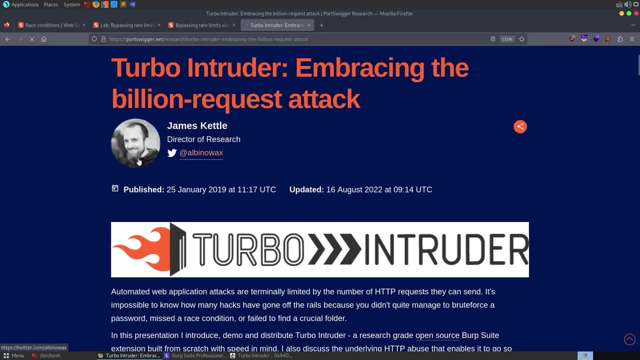 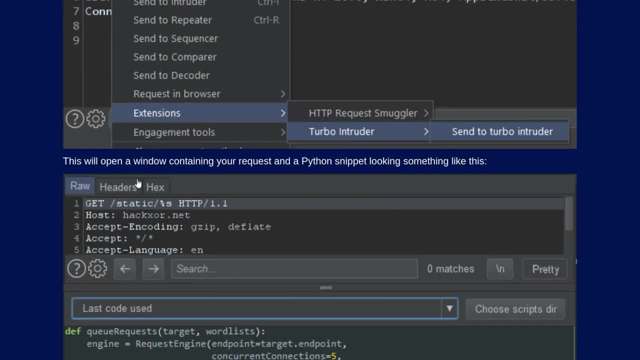 And if you want to learn even more about Turbo Intruder, You can check out this article- It's quite a few years old now- from James Kettle, But it talks a lot about how you can configure it, How it works And some of the cool features. 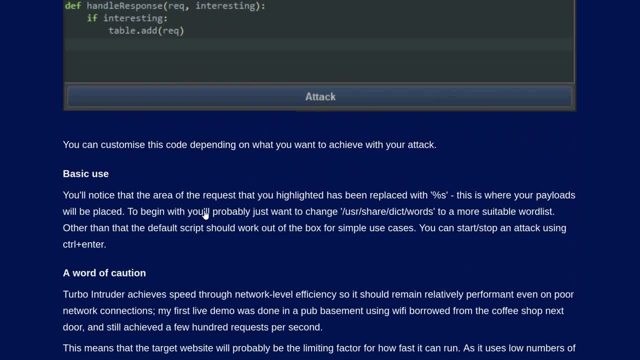 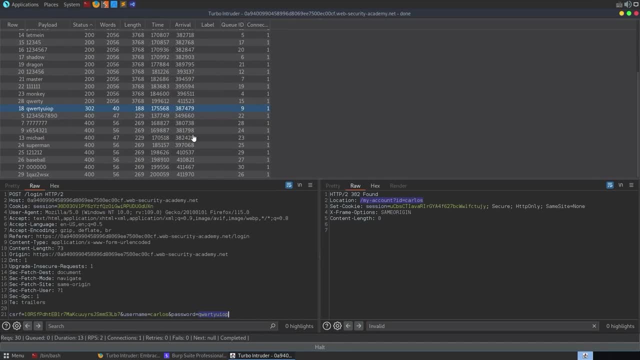 Something that we didn't yet show Is this handle response option. Let me see So. here's an example of Trimborium results. So in our case, You'll notice that it added every response to this table, But what we could have said here is actually: 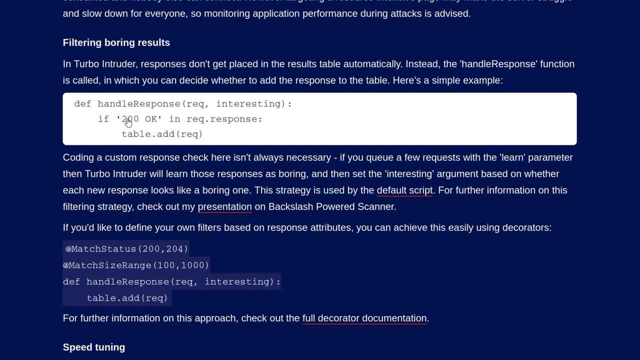 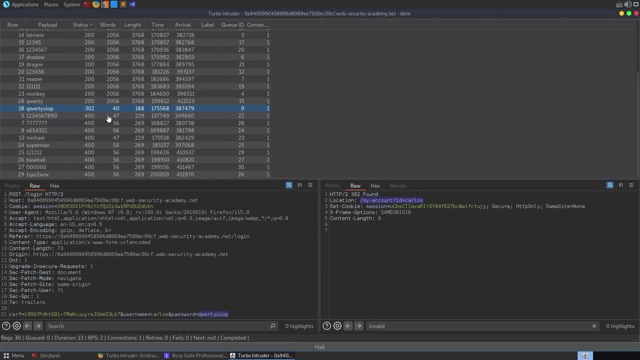 We only want to add responses if they are a 302. And that means that only the ones that have that successful login attempt. And you might think: How do we know it's going to be a 302?? Well, we just go and log in with the account we have the credentials for first. 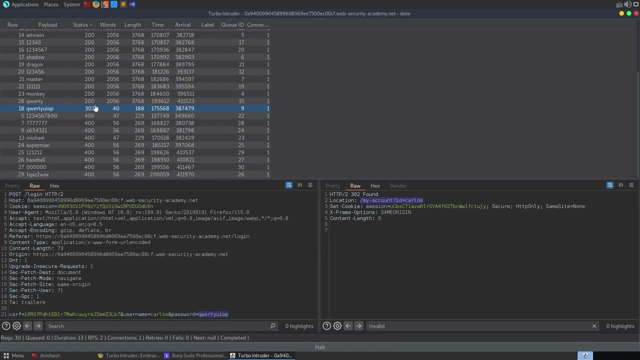 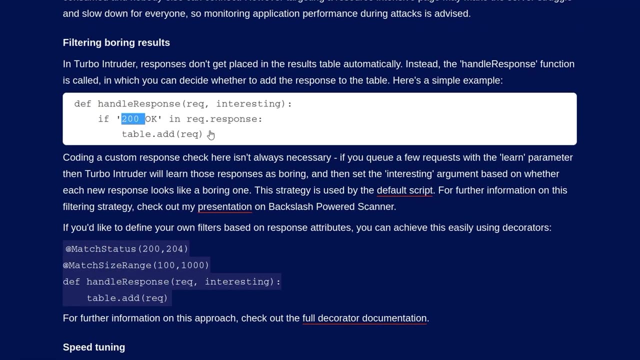 And see how it behaves. Does it come back with a different response code? Does it have something different in the response, Some text or something like that? So if this just came back with a 200, OK, But it had a string in it saying successfully logged in. 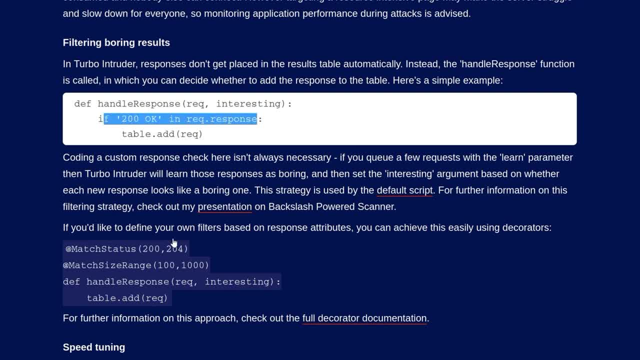 Then we would just update this accordingly And we can also filter on other attributes. So you can see, here We can say we basically only want to match responses that have a 200 or a 204 response code, And we can say that we only want to match responses that are within this range of sizes. 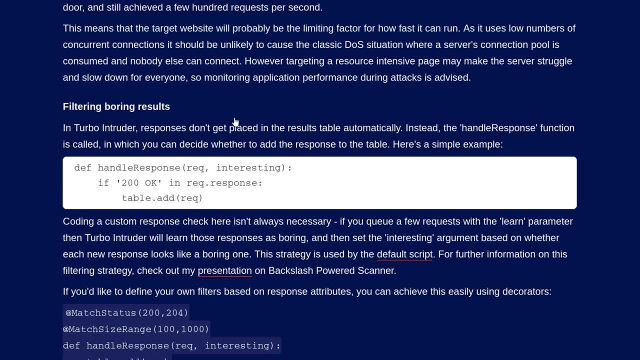 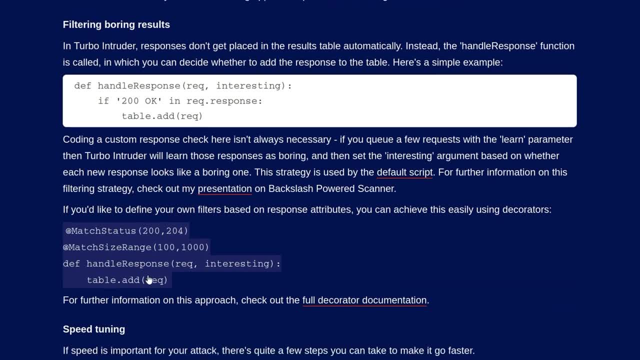 So that's important, because if you're doing this with a very big word list, A lot of requests, Then every one of those is going to be added to the table And it will eat up your RAM. So by filtering out responses that we're not interested in. 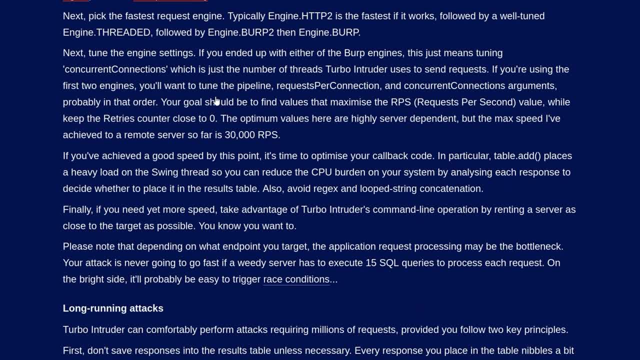 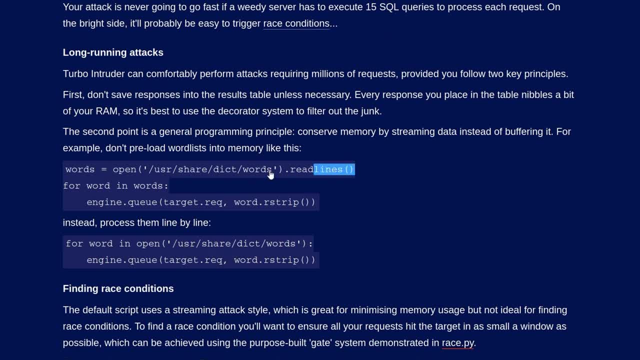 You can basically help with the performance. It also mentions that it's a good idea to loop through the words line by line, Rather than reading the whole word list And then looping through those words For the same reason. It's going to eat into your RAM. 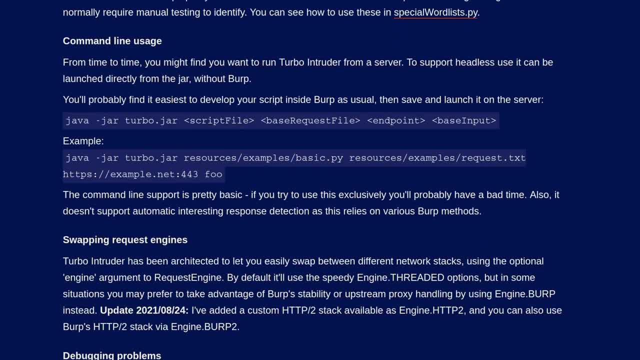 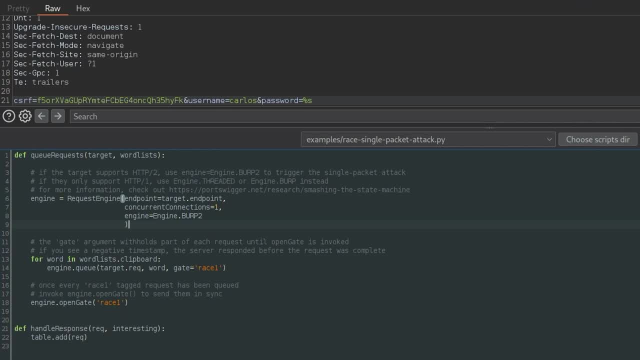 There's probably a lot of other cool things in this article Which I've forgotten about, But you can check this out in your own time. Let me just show one final thing. If we go back to our Turbo Intruder- So in this case we use the clipboard- 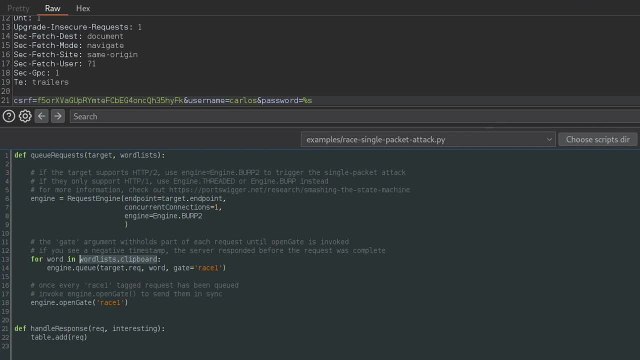 But what if we want to test a lot of passwords? Well, we might want to open up the word list here. So we could say, like, If we want to open up rocku, There we go, We provide the file path. The problem is rocku, as you may know. 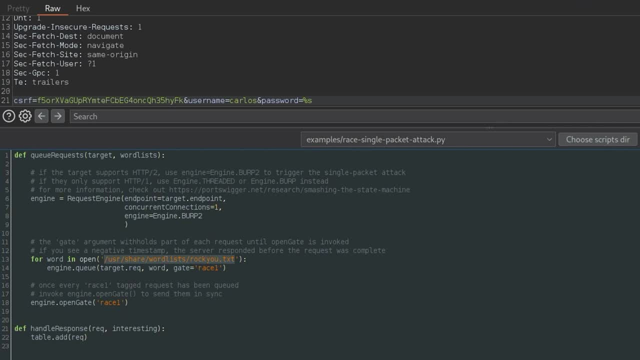 Has millions of passwords in it. So if we do this, Essentially what we're doing Is we're queuing those millions of passwords into requests And then we're going to open up the gate And send them all at once. Now, if we send more than 20 or 30 passwords at once, 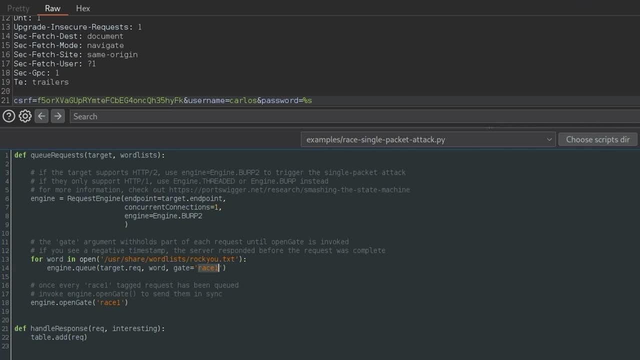 In this single packet attack, The others aren't going to get through. So in other words, The first 20 or 30 will come back and say Invalid password or correct password, But all of the requests after that Will come back and say that you've been locked out of your account. 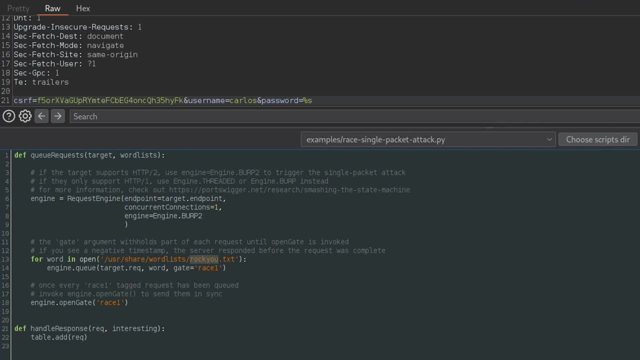 Which means we would need to do All of those millions of passwords again. So it makes no sense to send them all at once. In this case we might use a subscript, So we could say let's just do 0 to 20.. 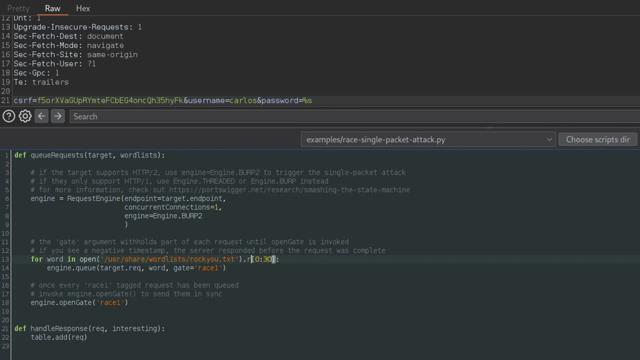 Or 0 to 30 on the first attempt, But to do that we also need to use that read lines, Which it did advise us not to do. But that will basically get around to that, So we could give this a go. I've actually relaunched the lab. 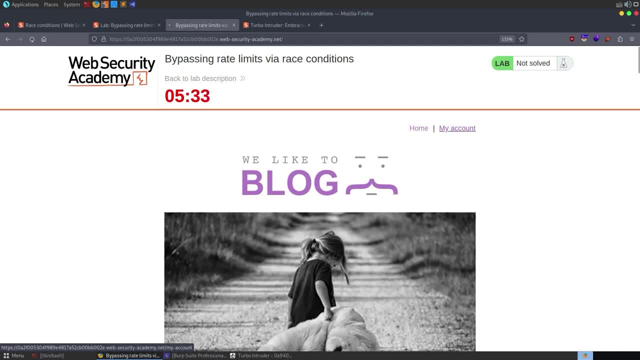 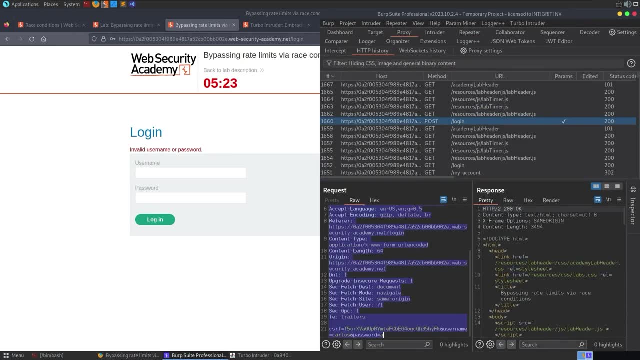 Which is still running. So if we go to our account And do Carlos, And then let's just go and grab that request, Take a copy of it, Go back to our turbo intruder, Set this to %s again And then we can go back. 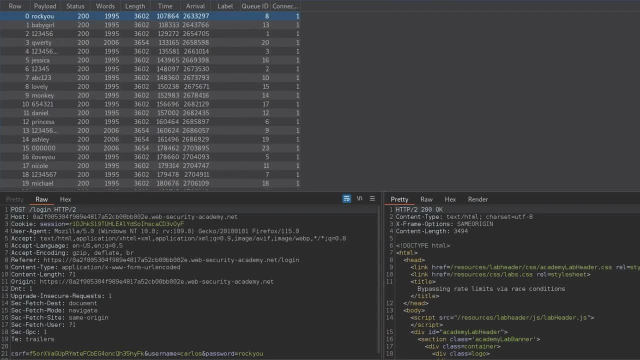 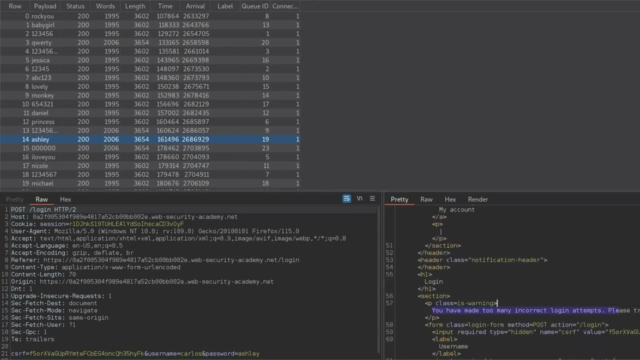 And then we'll click attack And there we go. So we get back to the 30 responses. Notice that some of them are 3654.. And that response size indicates That we've got too many incorrect attempts. So if we filter it by that, 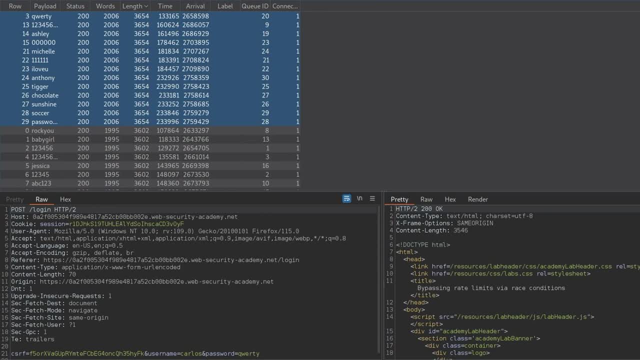 We'll see that actually, I think around 10 of those Failed to be tested. So it means we basically, Yeah, we only got 0 to 20.. And then after that The next 10 weren't tested, So we can go back. 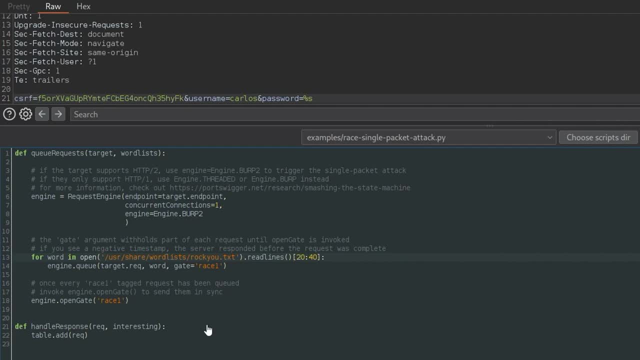 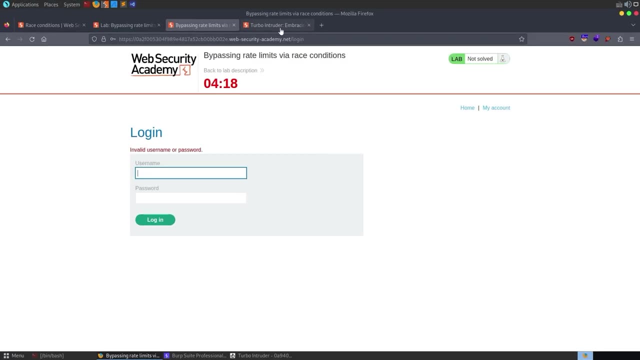 And then do from 20 to 40.. Oh, the other thing to mention Was the handle response. So at the moment this is set to, It takes in a request and interest in- And actually this was in the article as well. I forgot about that. 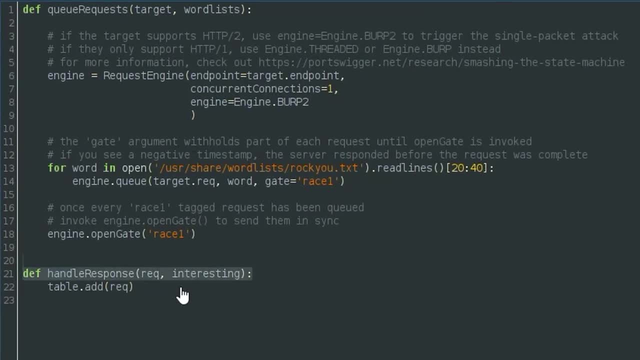 So the interest in? apparently It takes like a baseline Based on what responses look like, So that if you're getting a lot of responses With the same parameters It will stop adding those to the response table. I believe We'll only add it to the table. 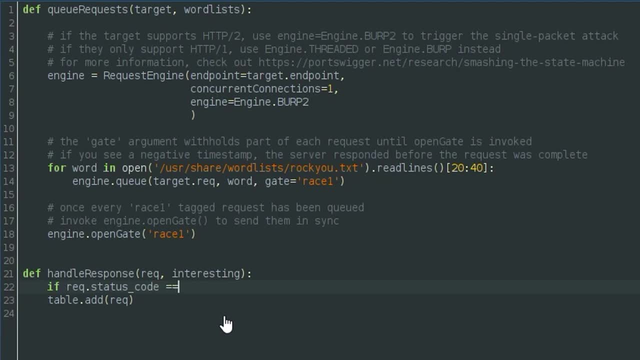 If the request Status code Is equal to 302.. Because we know that's what we're looking for. That's a successful login, So we could do that. Let me see whether our time has reset. We've got 25 seconds left. 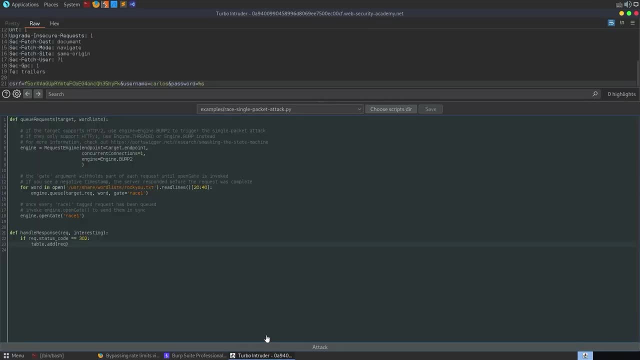 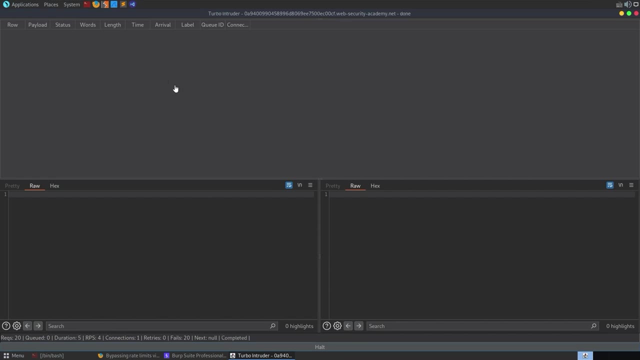 Okay, that should be the lockout reset. Let's go and try this. We'll click attack And now we're doing the next 20 passwords, But we're only adding them to the list If we get the. Okay, we've got 20 fails. 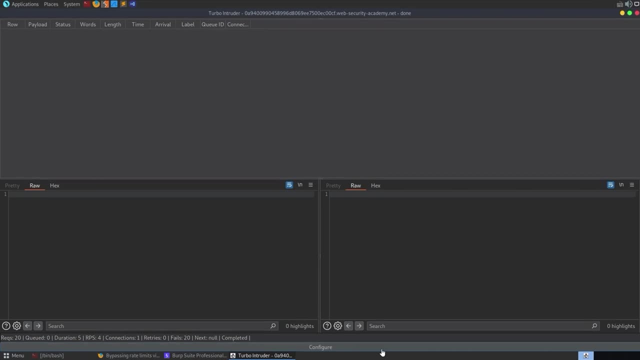 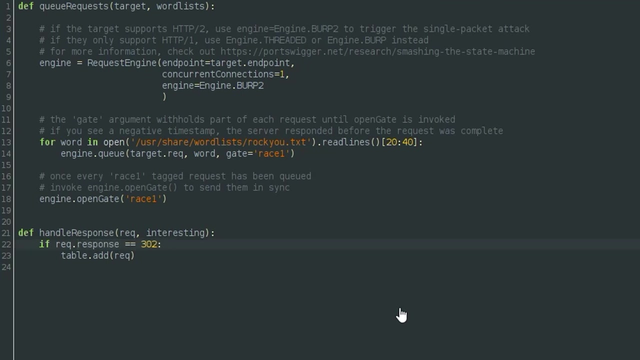 It didn't add them to the list Because none of them were 302.. So that's basically how we can do this. anyway, If we were to change this, We could say if the requestresponse. And then we could say contains: So we could say if: 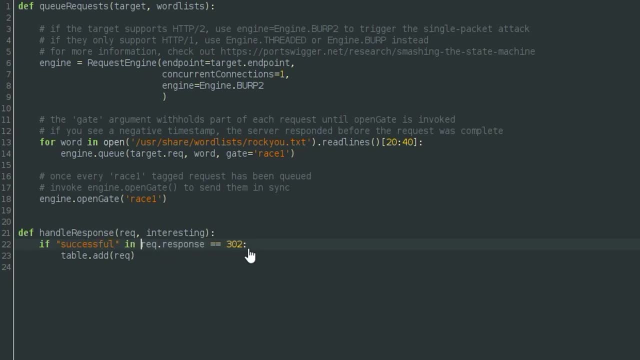 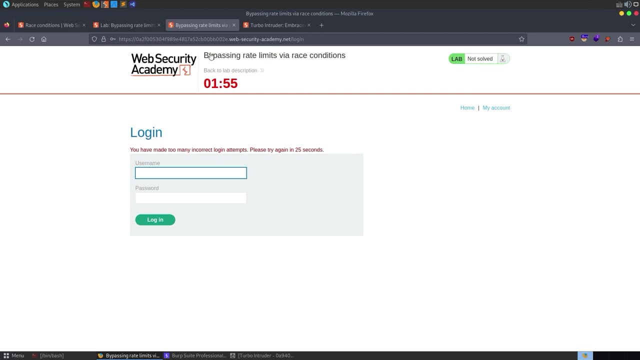 Successful In requestresponse, Then we want you to add it to the table, Or we could do the opposite of that. Anyway, to summarize, We have looked at how we can bypass rate limits Via race conditions And how we can brute force the credentials of users. 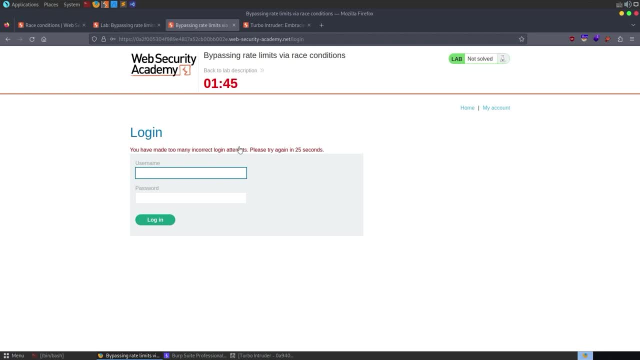 Unfortunately, Brute forcing of User passwords Or even username enumeration Is typically out of scope for bug bounty, So it's not going to help you too much there. But hopefully this education of getting into How race conditions work And how we can exploit them.